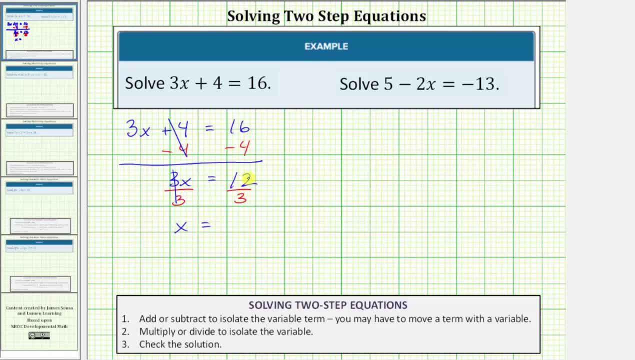 1 times x is x, So we have x equals. On the right side we have 12 divided by 3, which equals 4.. So x equals 4 is the solution. Well, let's verify the solution By substituting 4 into the original equation to make sure it makes the equation true. 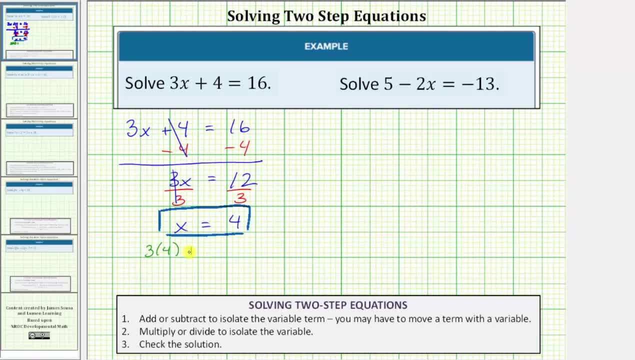 So 3 times x would be 3 times 4 plus 4 equals 16.. Simplifying the left side, 3 times 4 is 12.. So we have 12 plus 4 equals 16. And 12 plus 4 is 16.. 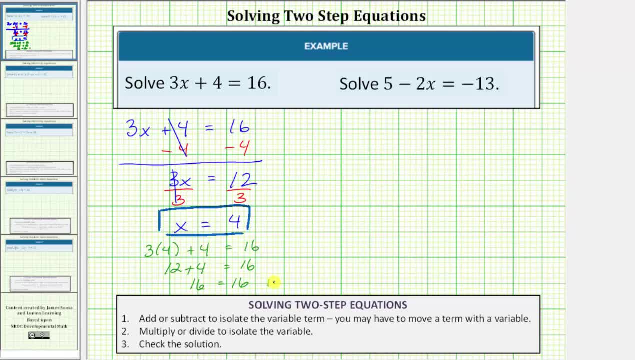 And therefore this simplifies to: 16 equals 16, which is true, Verifying the solution is correct. And now let's look at the second equation, which is: 5 minus 2x equals negative 13.. Again, the solution is the value of x that satisfies the equation or makes the equation true. 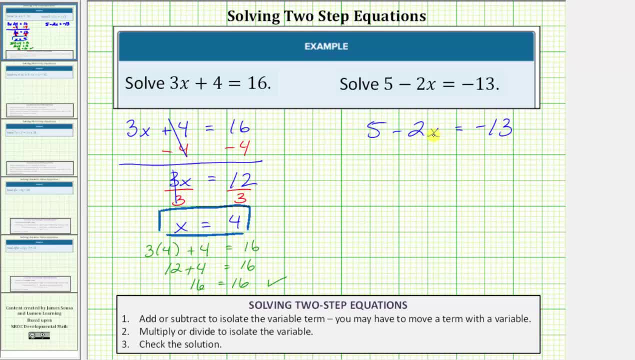 Which means the solution is the value of x. that makes 5 minus 2 times x equal to negative 13.. The first step is to add or subtract, to isolate the variable term. Here the variable term is negative 2x And therefore we want to undo this positive 5 by subtracting 5 on both sides of the equation. 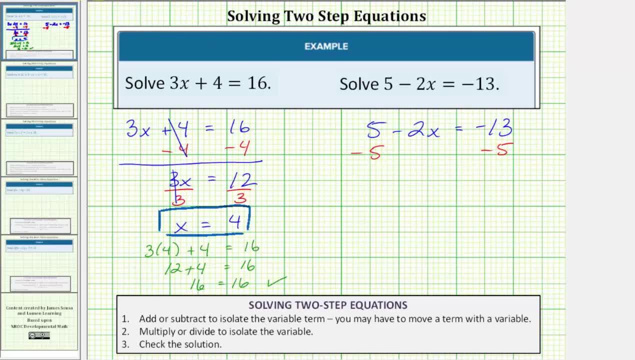 And now we simplify both sides of the equation. Notice on the left side, 5 minus 5 is 0. That's why we subtracted 5 on both sides of the equation. So the left side simplifies to negative 2x. 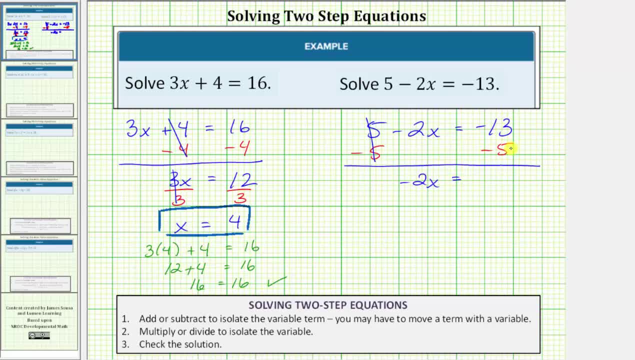 So negative 2x is equal to negative. 13 minus 5 is equal to negative 18.. Second step is to multiply or divide in order to isolate the variable and solve the equation. Negative 2x means negative 2 times x. So to undo this multiplication, the next step is to divide both sides by negative 2.. 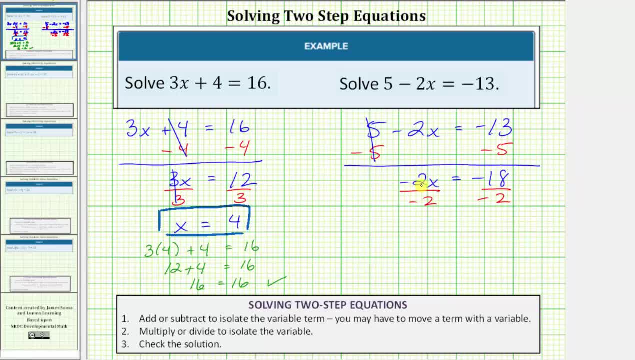 Now we simplify both sides. Negative 2 divided by negative 2 is equal to 1.. 1 times x is x. So we have: x equals negative. 18 divided by negative 2 is equal to positive 9.. So the solution to the equation is: x equals positive 9..